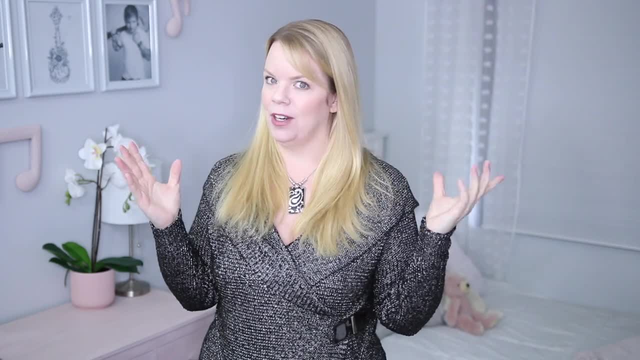 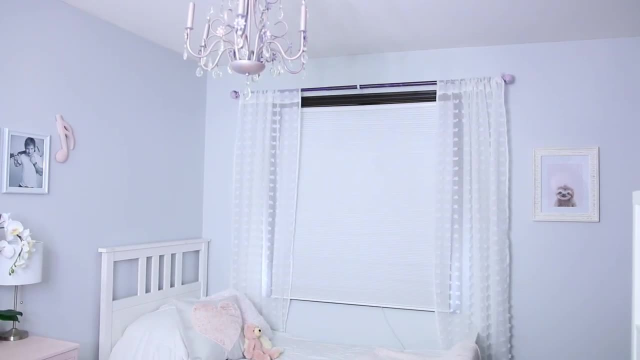 walls herself. So hopefully she loves it enough or hates painting enough to never want to have her room redone again. So we did the whole room in just a day. We're using a lot of the things we already had, but I wanted to share the organization with you because this is one of the number one. 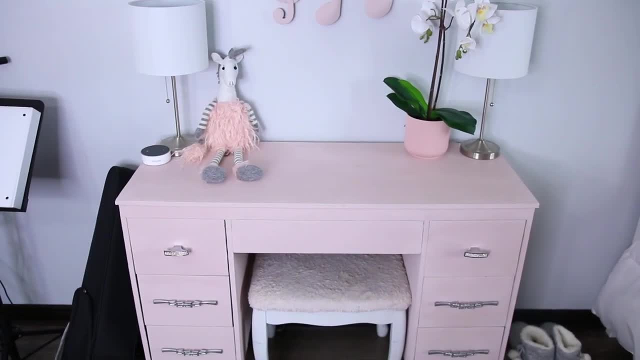 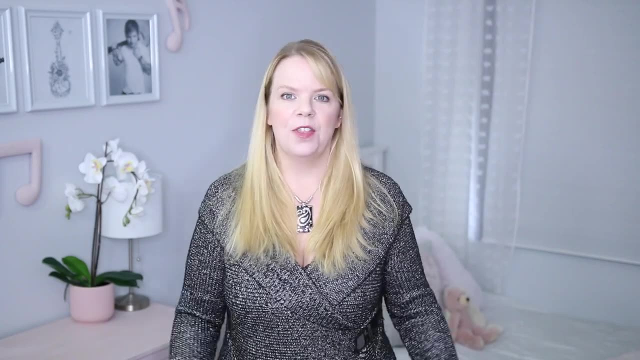 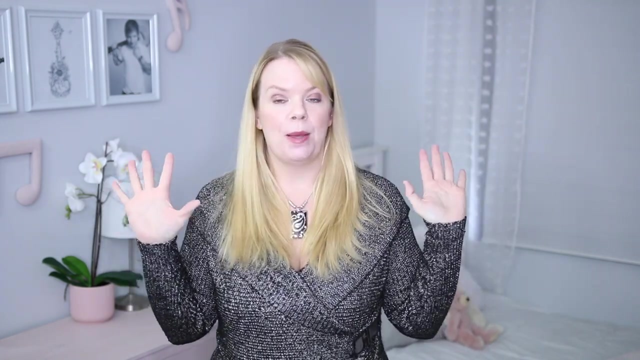 questions that I get: How do you organize a kid's space so it stays clean and tidy all the time? So I'm going to share my top five tips with you right now. The first tip I've said literally a thousand times, I know, but I'm saying it because, honestly, it's the greatest tip for kids bedrooms ever, And that 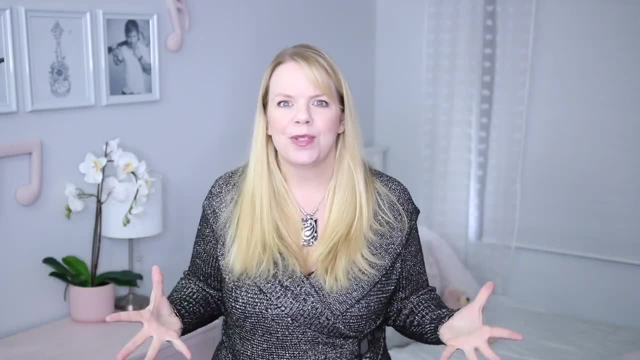 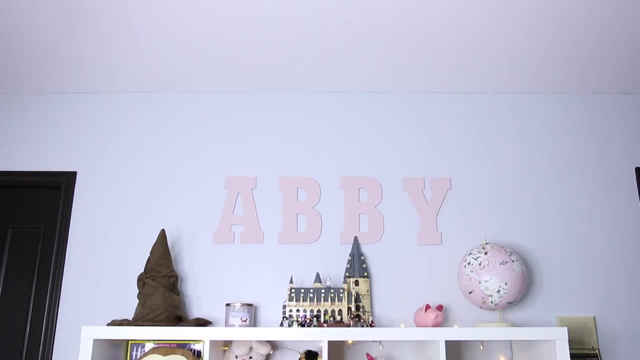 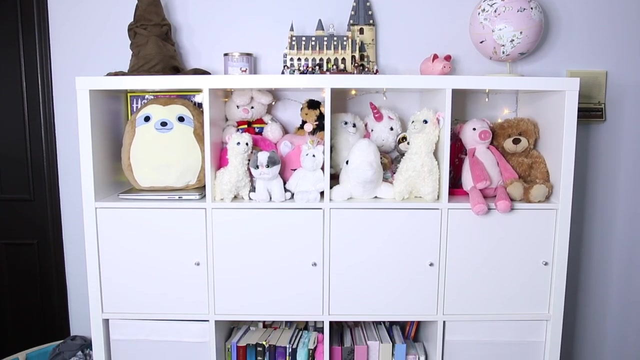 is ditching the dresser. Kids just shove clothes into dressers anyways. They don't hold a lot of clothing. They take up floor space instead. opt for a calyx shelf from Ikea. The bins hold so many clothes. It's easy for kids to find what they need to put it away. But the best part is because it. 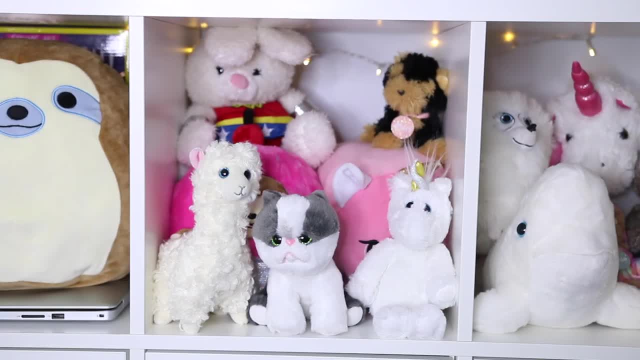 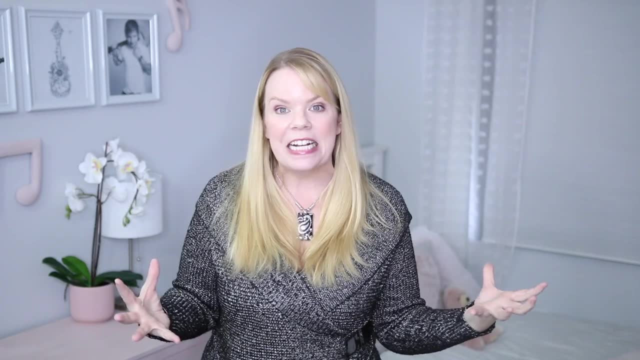 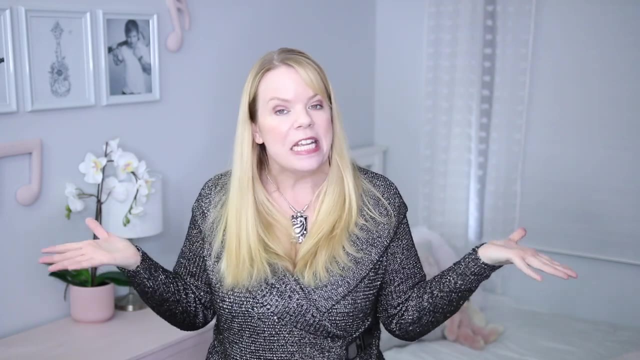 takes advantage of that vertical space. You have spots for their stuffed animals, their toys, their Lego, their books. You can hold so many things and it doubles as a dresser, which is a win-win: Less clutter and less floor space taken up. You need one of these shelves in. 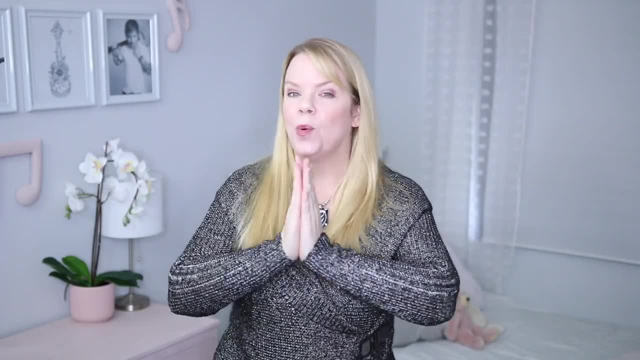 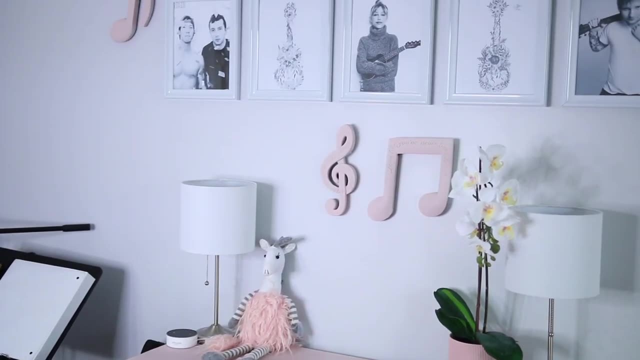 your kid's room. If you do have a kid's dresser or a desk, it's so important that you use drawer dividers. Kids are macro organizers so they're like dumping and tossing and things can get out of control fast. But with some dollar store drawer dividers or little bins inside your closet. 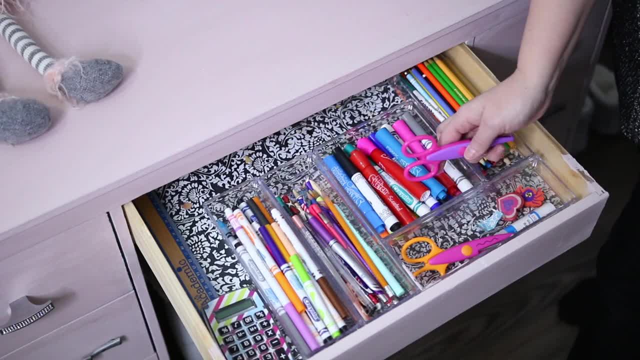 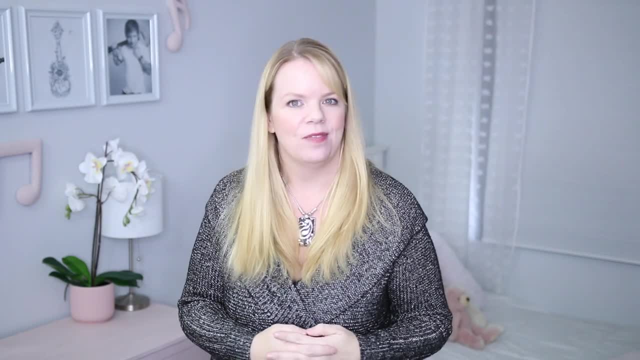 or inside drawers. they're going to keep it so much tidier because their brain sees the little dividers and they toss them into their actual home. Definitely have to give this a try. If your kid's room is short on space, you've got to try this. under the bed rollout It's. 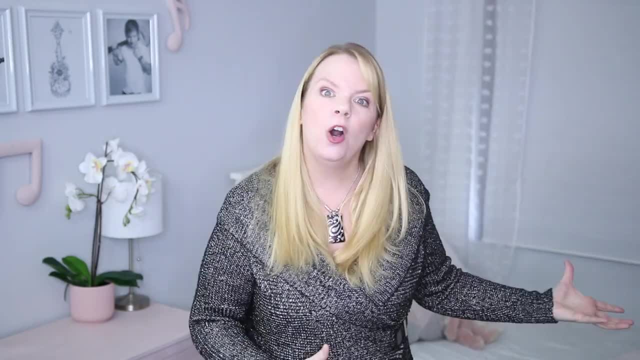 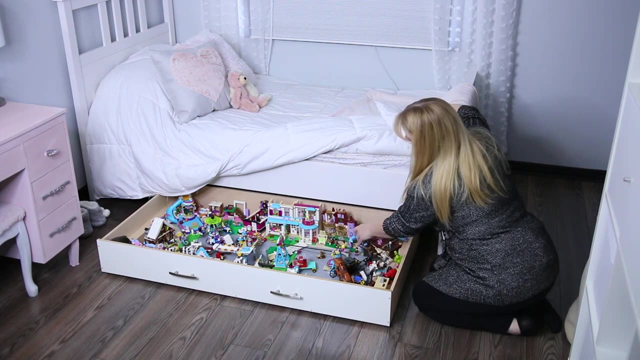 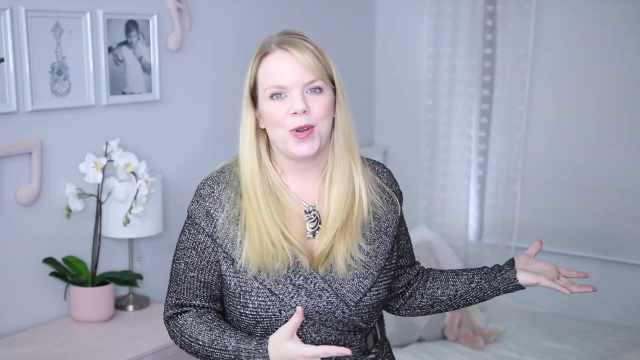 definitely maximizing the space. It's the perfect spot for Lego or train sets or Barbies or whatever your kids have an abundance of. They can roll out this under the bed storage, play, make a mess and roll it back under when they're done. If you don't need extra toy space, you can use under bed. 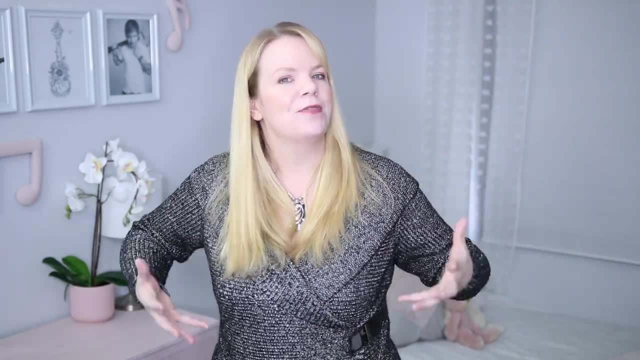 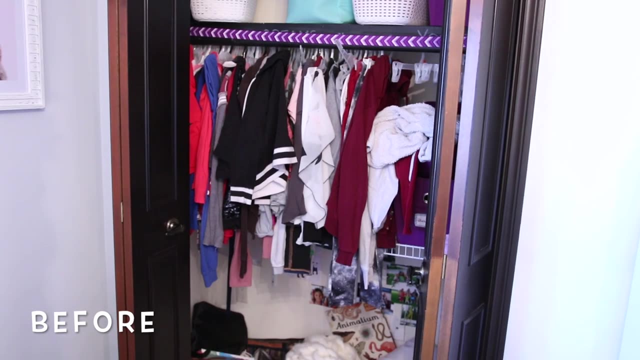 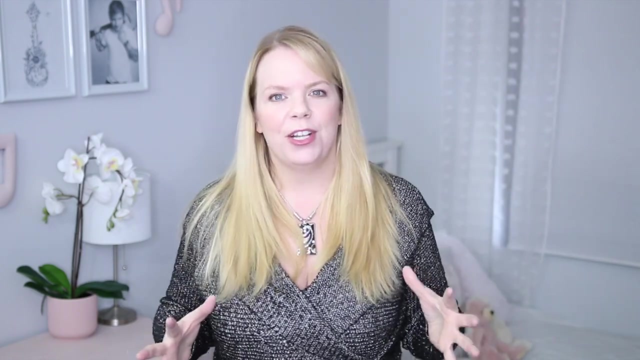 storage for off-season clothing or whatever extra stuff that your kids have. Next, it's so important to declutter your kid's closet Every single year. your kids will outgrow clothing and they will outgrow toys, and yet they're always shoved in the closet not being used. So every single year, 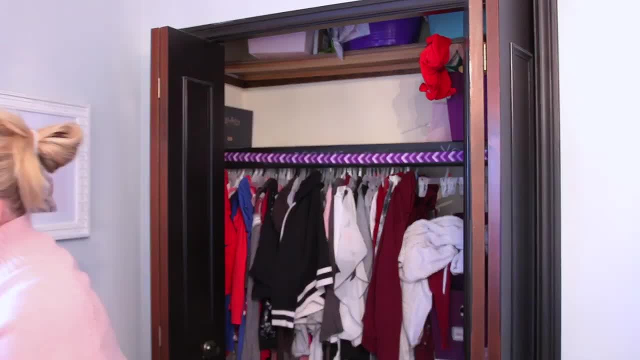 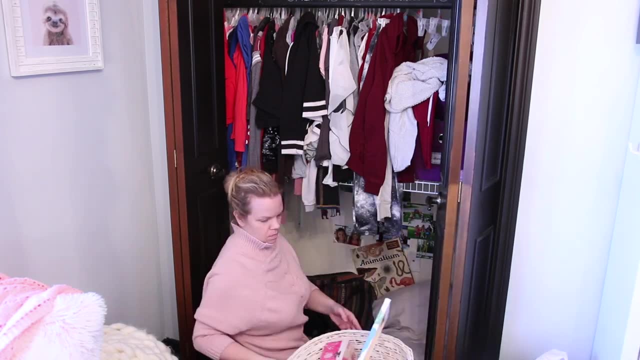 you have to do a big purge of your kid's closet. This means taking everything out, Deciding what they want to keep, deciding what they don't use and packing it up to go. I know what you're probably thinking. Your kids are reluctant to get rid of things. All kids, They. 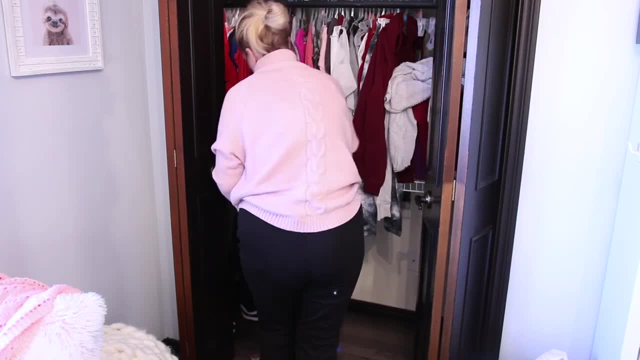 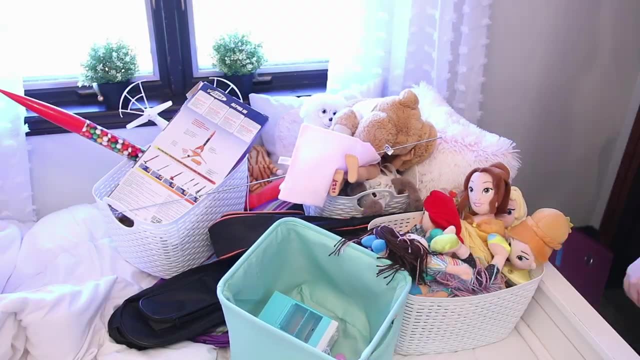 hate purging. So a really quick tip is for you to go through without them, Decide what they're not wearing and you know what they're not using, but let them have veto rights so they can come in, look at the box in the bag and pick a few things to keep. It's always much easier to. 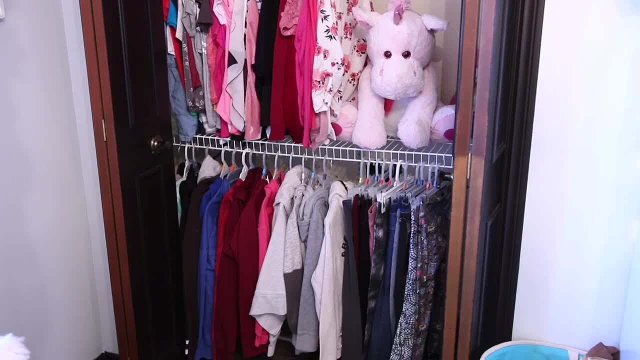 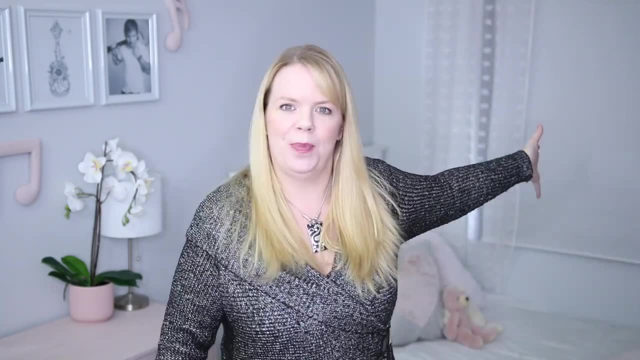 decide what you want to keep than it is to decide what to let go of. Last but not least, I really want to encourage you to use what you have. I know I said you should buy a shelf and under bed storage and drawer dividers for your kid's desk, but the truth is 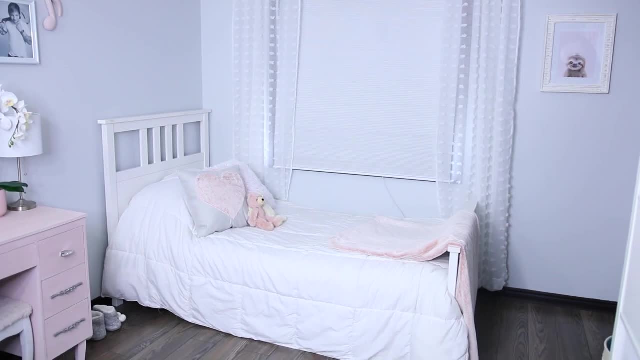 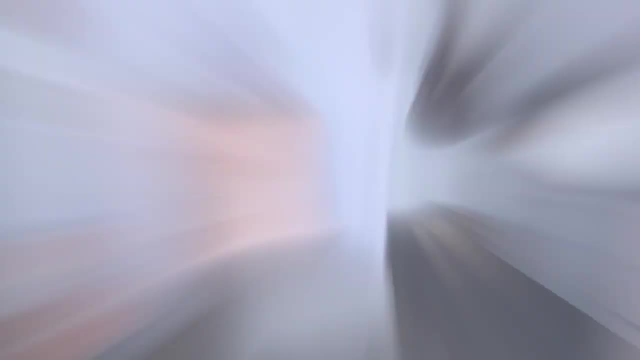 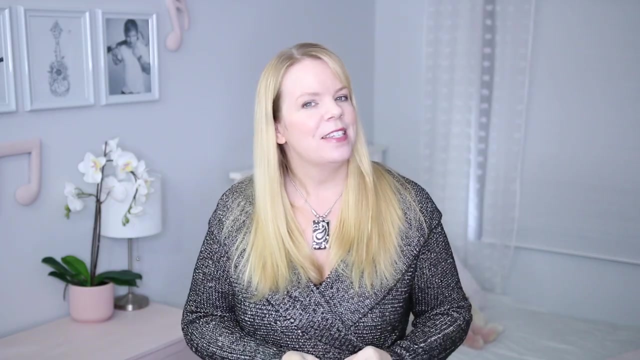 you can organize and declutter using what you already have. No need to go out and buy pretty matching bins or all matching hangers. Use what you have, Maybe rearrange furniture for better flow. Definitely declutter and get a little creative. You don't have to spend time or money. It's all up to you to decide what you want to keep and what you don't want to use. I know I said you should buy a shelf and under bed storage and drawer dividers for your kids' desk, but the truth is you can organize and declutter using what you already have, No need to go out and buy. 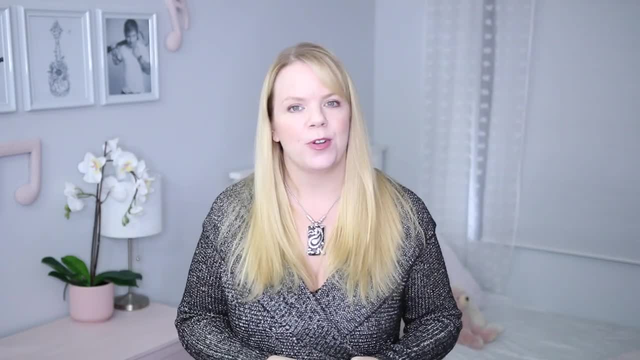 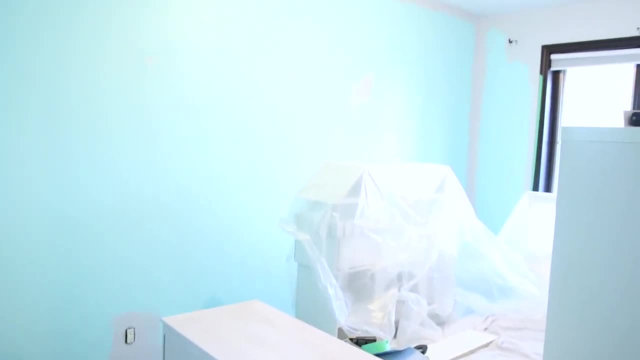 to have a beautifully organized and tidy kid's bedroom. When we made over Abby's room, the only thing we actually bought was new pillows and a can of paint. Everything else was reused. I love reusing dollar store picture frames. just printing pictures off the internet. It changes. 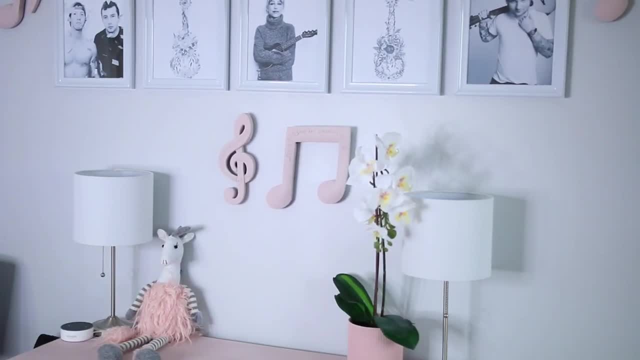 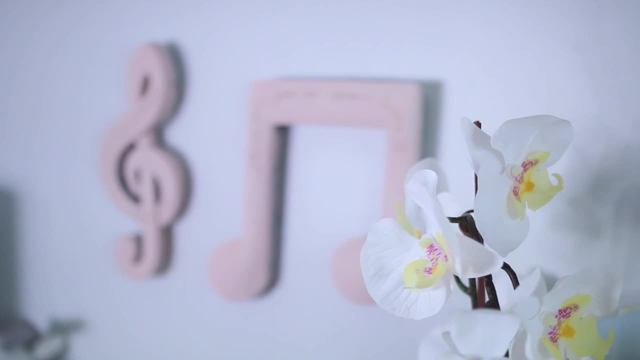 the whole feel of the space without spending any money, And one can of Annie Sloan chalk paint recovered things like the desk and the little music notes and Abby's name on the wall. So you don't have to spend a lot of money on that And I think it's a really good idea to have a